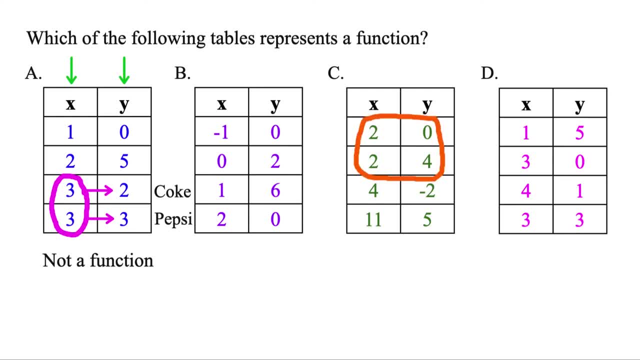 So which of these other ones are also meant to be a function? Well, C, because if we press button 2, we get two different things out, No good. Or that last one: You push 3,, you get a Twix. You push 3,, you get a Snickers. 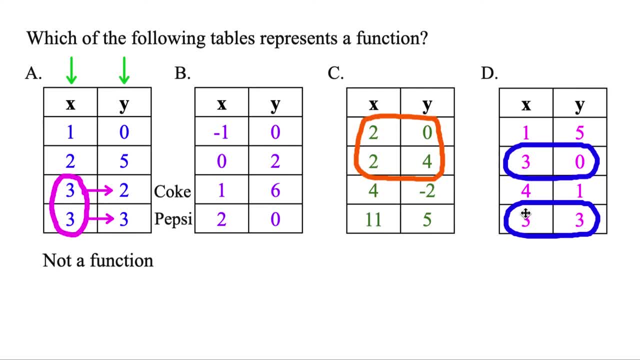 Well, that's fine, but we wanted a Twix, So B is the only one that is not messed up. That's our function. So that's how I recommend: find all the ones that are messed up, and then whatever's left is a function. 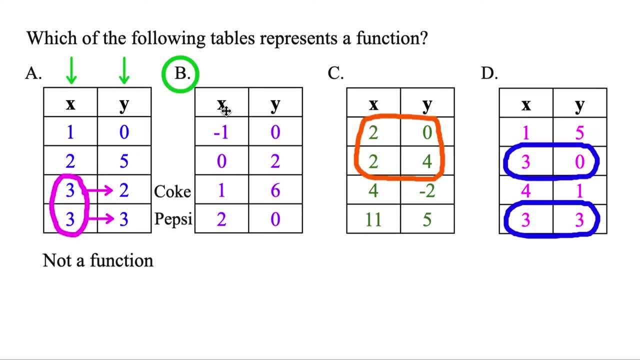 This is the one that's good. Or you could always think: if the X's are all different, it doesn't have a chance to be messed up, So that one must be good. X's don't repeat. That's the thing we're looking for. 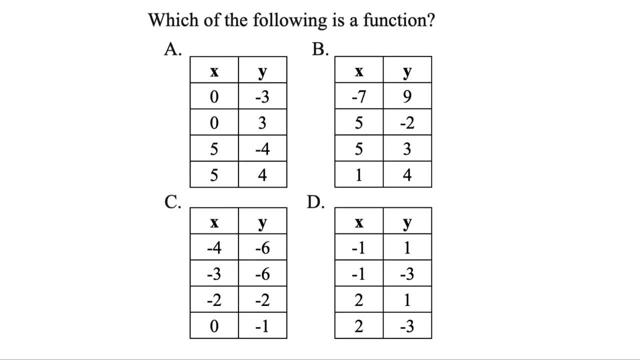 Okay, feel free to pause and practice with this one. Let's check it out. A: two buttons are messed up. That's out B button 5. That's jacked up. And D: this is just a minefield of broken vending machines. 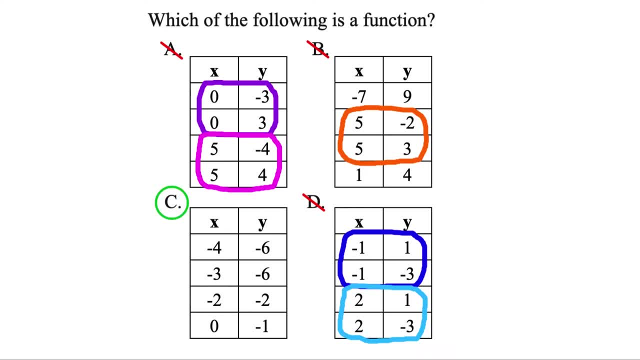 But, lucky for us, one left over. That's the function. Nothing repeats, Therefore it's consistent. Now, is it okay to have the same Y value in two spots? Definitely, It's just stocked with the same thing in two different locations. 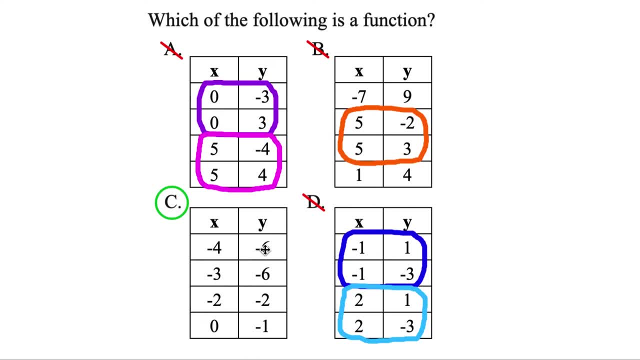 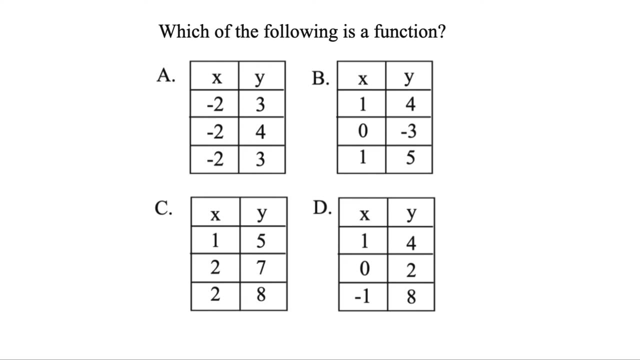 But you've seen that before You press one button, you get Pop-Tarts. Or you could press another button and get Pop-Tarts, but nothing's inconsistent, It's just giving the people what we want, So we're good. And one last one here. Feel free to pause. 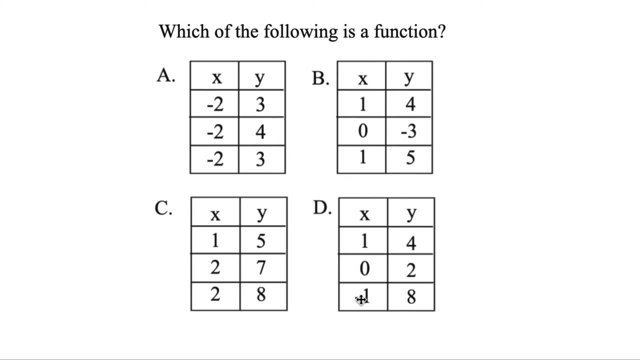 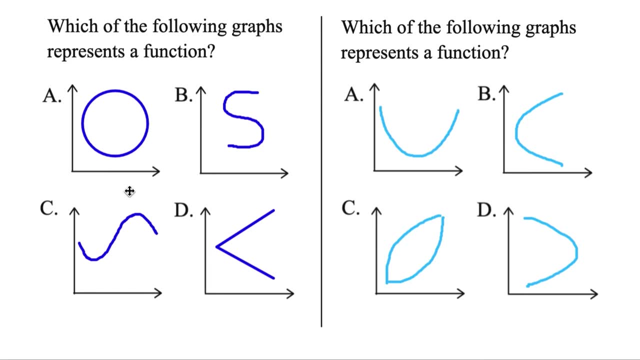 You know it: D different X's. We're good, That's our function. Okay, how do you determine a function if you're given graphs? All you need to do is draw a vertical line Anywhere on the graph And it should only hit once. 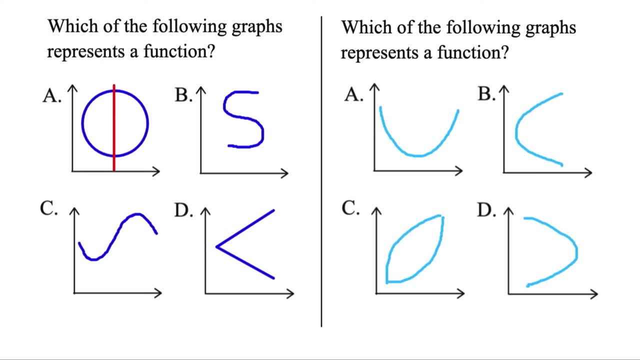 This one hits twice, Not a function. The next one: vertical line That hits three times, That's no good. But C that hits once, That's our function, Because D that hits twice, That's out. So look for the one. no matter where you draw the vertical line, it's always just going to hit once. 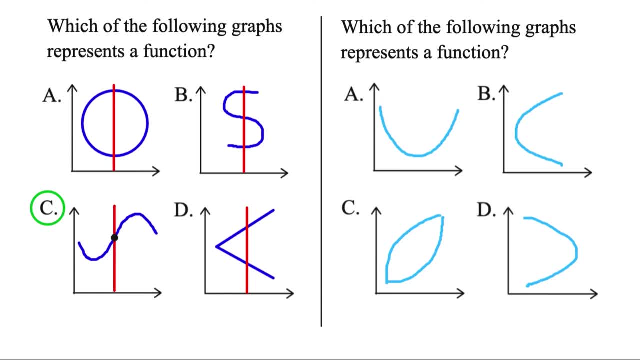 But why is this a function? Well, let's label this point. The bottom is usually time. Let's say at 9 am. however high that graph goes is the temperature. Therefore, at 9 am there can only be one temperature. 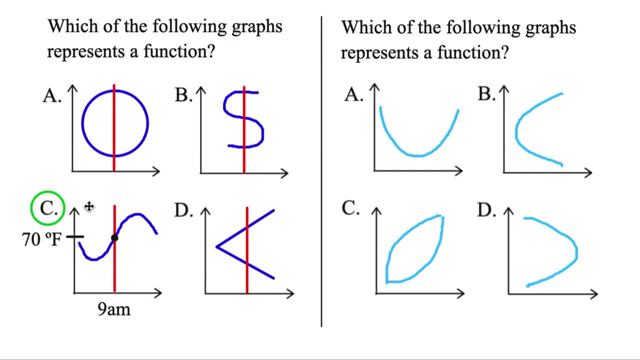 We'll call it 70 degrees, But the issue is with A, because that would say at 9 am it's 20 degrees and it's 100 degrees at the exact same time. Not possible, Not a function. So functions will always model things that happen in real life there. 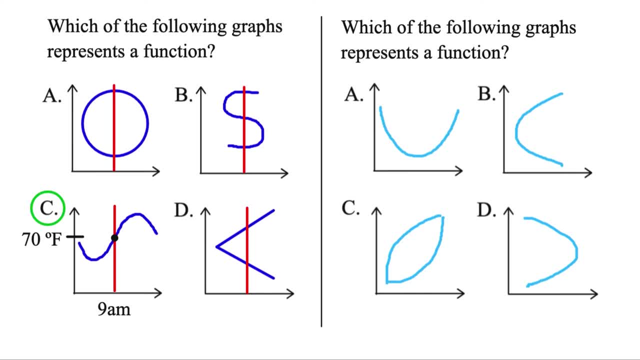 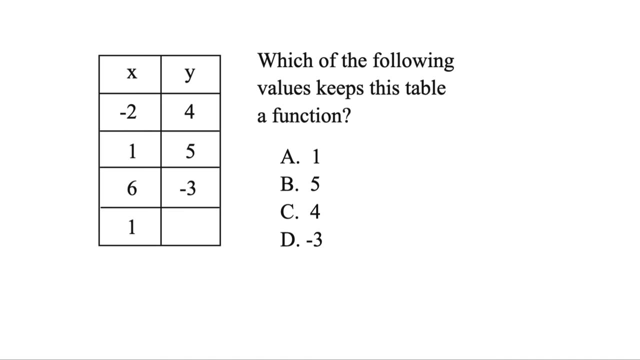 Feel free to pause for that last one there. And it just so happens the first one we check, anywhere we draw a vertical line hits once. That's our function. Which of the following values keeps this table a function? Now, earlier I was saying you don't want the x's to repeat. 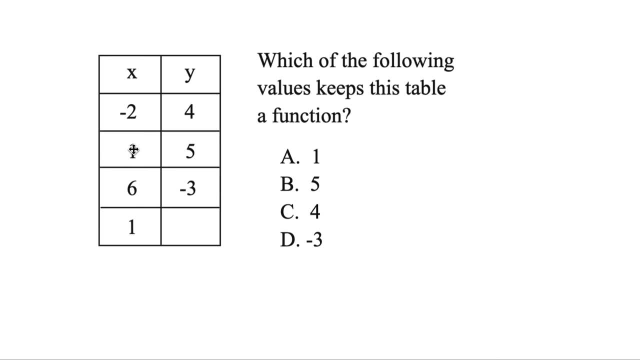 But what if they do? Well, last week we had a bad breath day, We push button 1. We got some trident gum. But then next week same thing: bad breath day, Push button 1. We want some more trident. 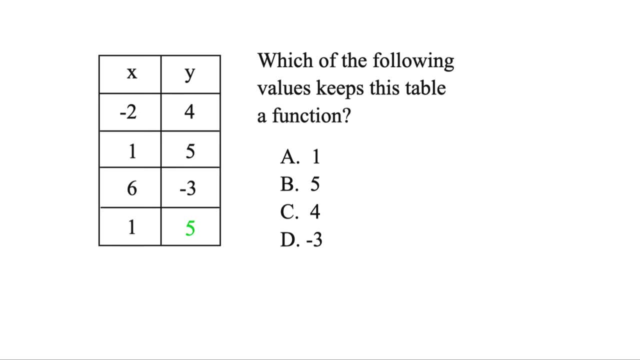 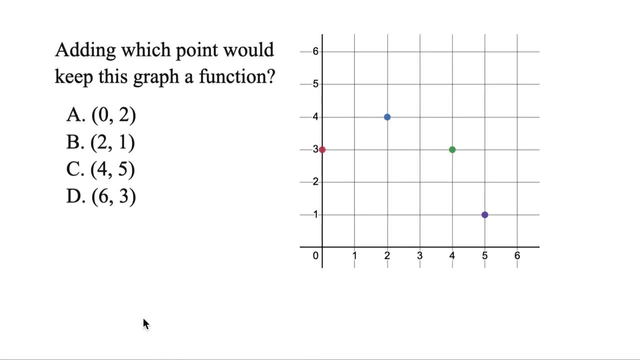 We want to get the same y value. That'll keep it consistent, That'll keep it a function. That's our answer. And one last one: Adding which of these points will keep this graph a function? The main thing is, we just don't want points stacked on top of each other like we had over here. 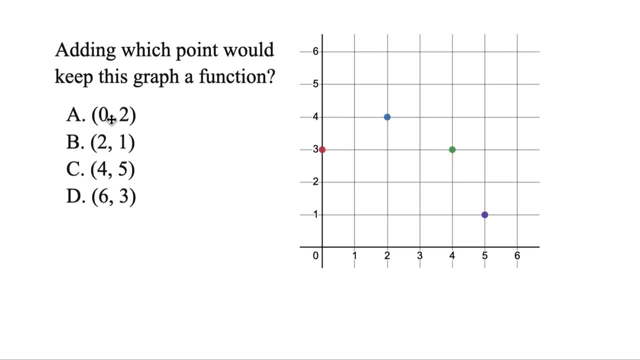 So let's plot these one at a time: 0,, 2.. We'll always start at the origin. The first number is to the right. We're at right: 0. Up, 2.. Put our point, There we go. 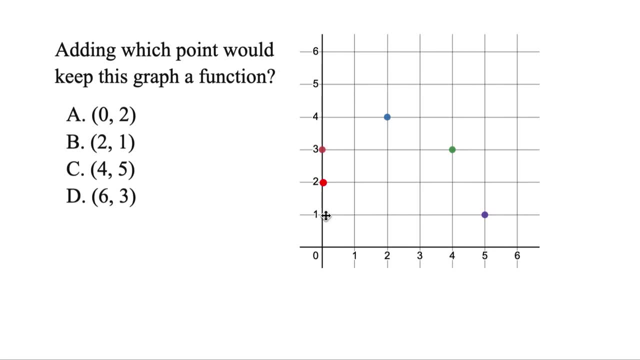 But unfortunately those are stacked. We draw a vertical line Passes through twice. That is not a point we want. Let's get rid of it. Okay, let's try the next: Right, 2. Up, 1. Start at the origin. 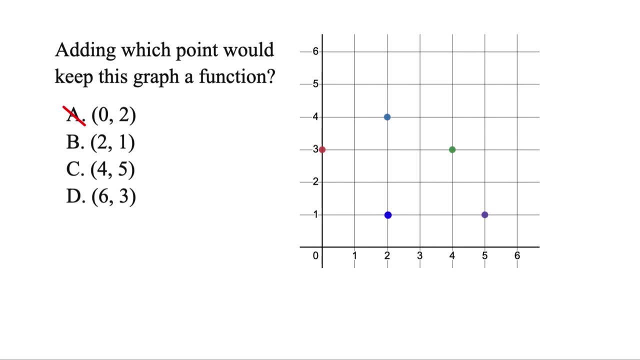 2 to the right Up: 1. Put our point, Ah, but once again that one's also stacked. That's no good. And then 4 to the right Up, 5.. Right, 4. Up, 5.. 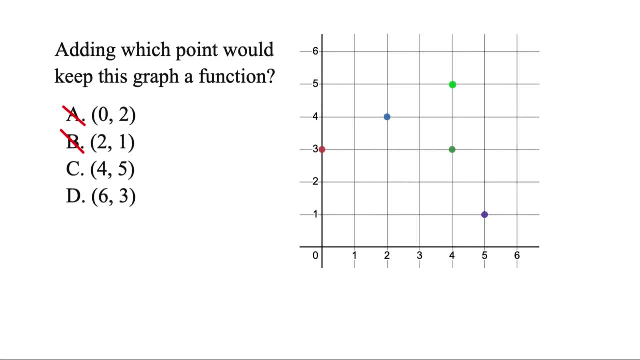 But we can see that one's also stacking, So that's no good either. So it has to be that last one. 6 to the right Up, 3. That'll give everything its structure. That'll give everything its space. That'll make it a function. 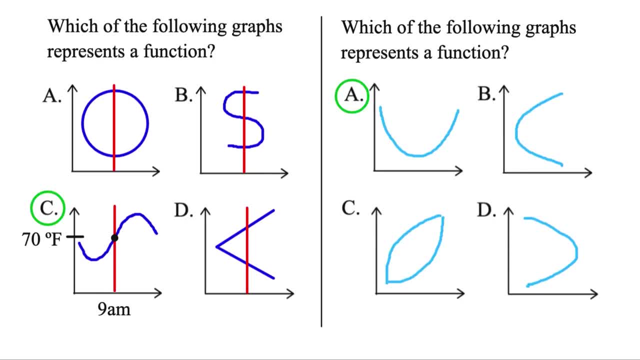 So these are the main types that show up on the GED. You got these. We'll see you in the next video- Toodles. 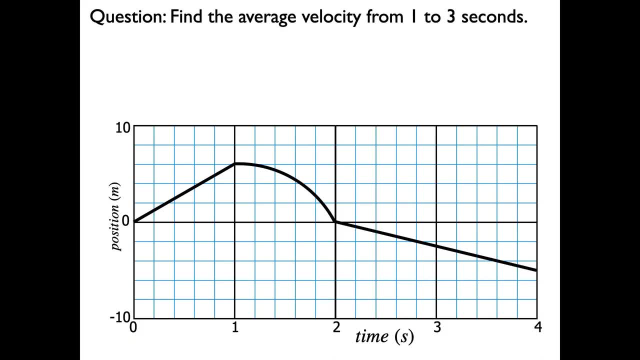 This video is going to show you how to find the average velocity on a position versus time graph. The question we're going to use to do this is to find the average velocity from one to three seconds, So what I need to do is figure out where I am on the curve at one and three seconds, So at 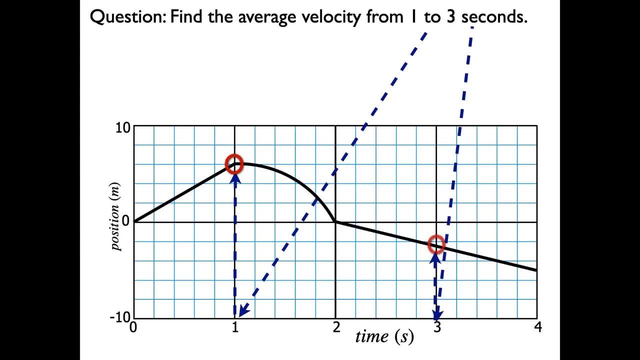 one second I'm there on the curve and at three seconds I'm right here on the curve. Now recall that the slope on this graph is the velocity. So what I'm going to do to find the average velocity is I'm going to draw a line between the two points at one second and three. 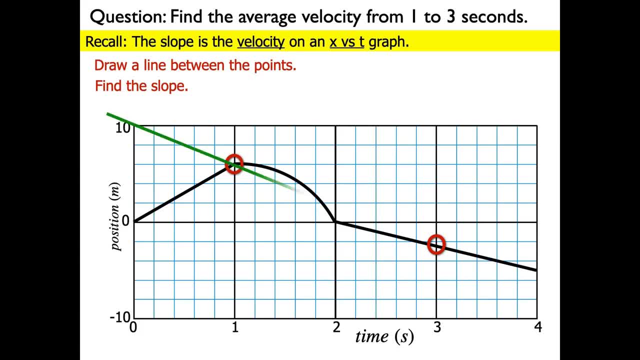 seconds, and then I'm going to find the slope of that line. So here's my line connecting my two dots. Now, at one it's kind of nice: it's in the corner of a square, so it's going to be some easy information to get. but at three seconds it's a little bit more difficult. So I'm going to follow. 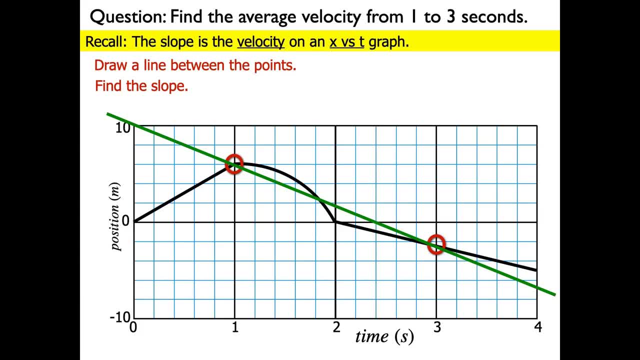 the green line down and I can see that at 3.8 seconds it covers the corner of the square. So that's the point I'm going to use in my calculations. So I'm going to start by using the one second, because it goes to the corner of the square. 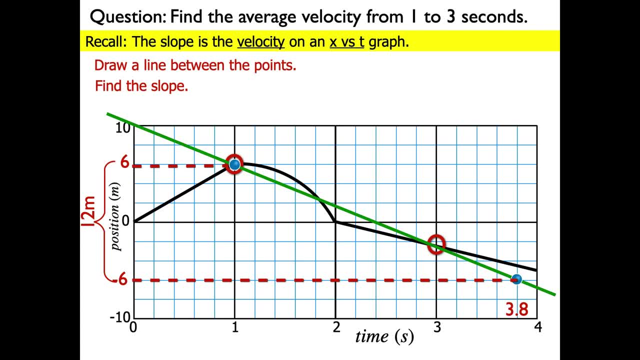 So that means that the rise is going to be 12 meters and the run is going to be the difference to my two points along the horizontal axis, which is going to be 3.8 minus 1 or 2.8 seconds. So the average velocity which